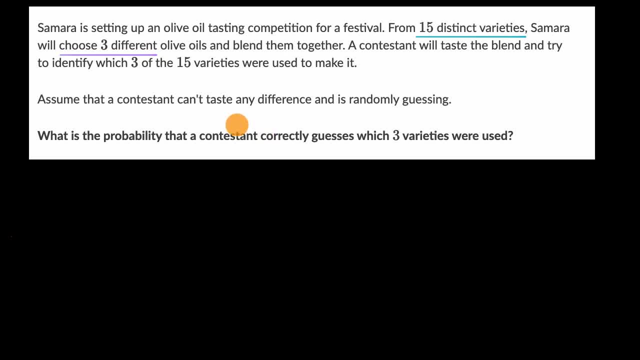 And anytime we're talking about probability and combinatorics, it's always interesting to say: does order matter? Does it matter what order that Samara is picking those three from the 15?? And it doesn't look like it matters. It looks like we just have to think about. 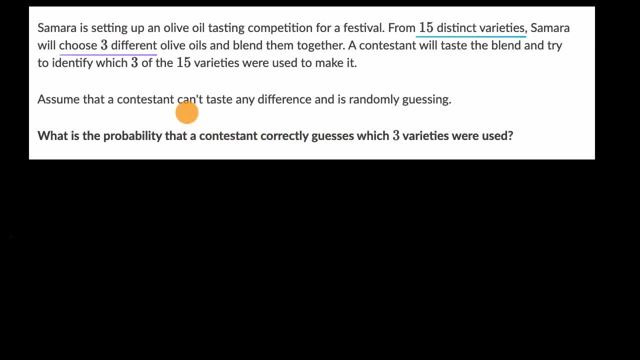 what three they are. It doesn't matter what order- either she picked them in or the order in which the contestant guesses them in, And so if you think about the total number of ways of picking three things from a group of 15, you could write that as 15 choose three. 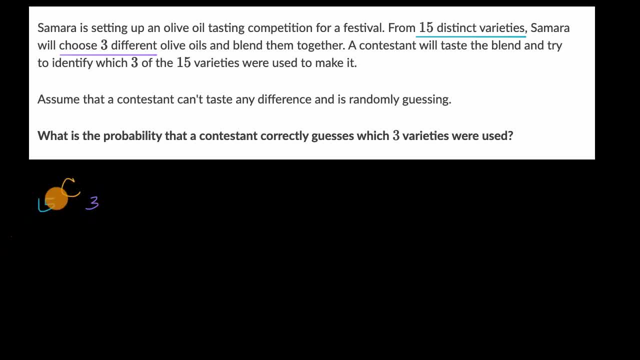 You could write that: as 15, choose three. You could write that as 15 choose three. Once again, this is just shorthand notation for how many combinations are there? so you can pick three things from a group of 15.. So some of you might have been tempted to say: 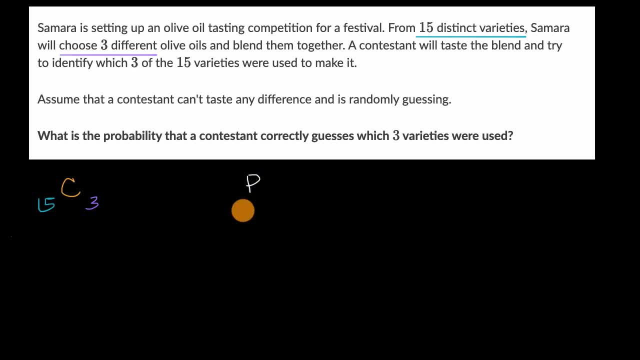 hey, let me think about permutations here And I have 15 things And from that I wanna figure out how many ways can I pick three things. that actually has order mattering, But this would be the situation where we're talking about the contestant. 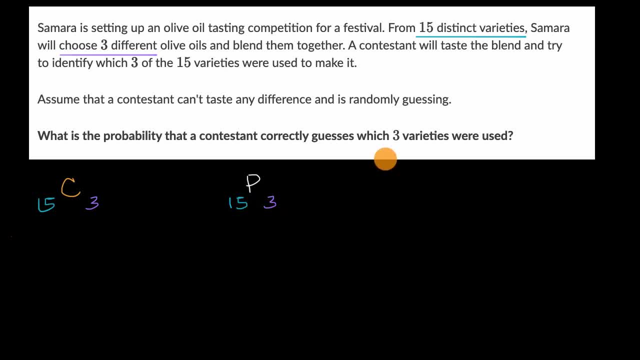 actually having to maybe guess in the situation, guess in the same order in which the varieties were originally blended, or something like that. But we're not doing that. We just care about getting the right three varieties. So this will tell us the total number of ways. 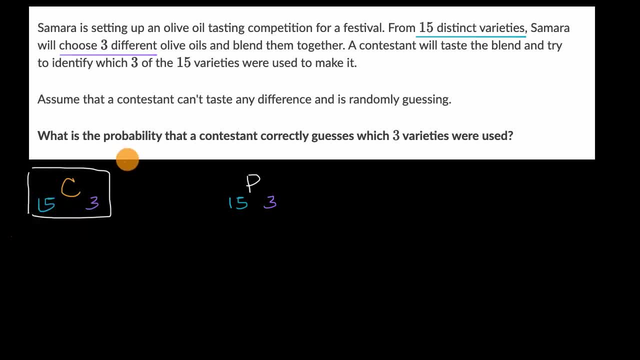 that you can pick three out of 15.. And so what's the probability that the contestant correctly guesses which three varieties were used? Well, the contestant is going to be guessing one out of the possible number of scenarios here, So the probability would be one over 15, choose three. 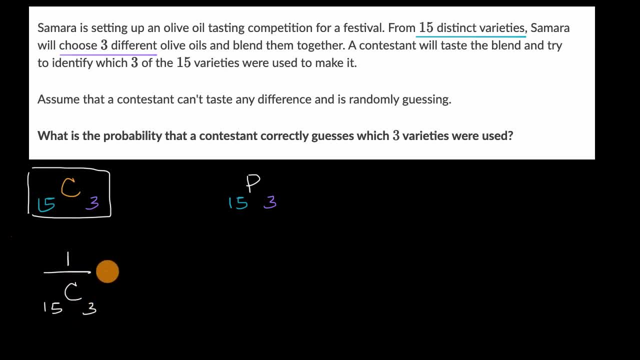 So the probability would be one over 15, choose three. So the probability would be one over 15, choose three, And if you wanted to compute this, this would be equal to one over. Now, how many ways can you pick three things from 15?? 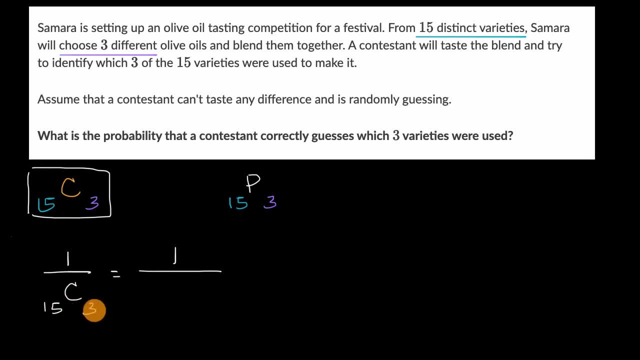 And of course there is a formula here, but I always like to reason through it. Well, you could say: all right, if there's three slots, there's 15 different varieties that could have gone into that first slot, And then there's 14 that could go into that second slot.